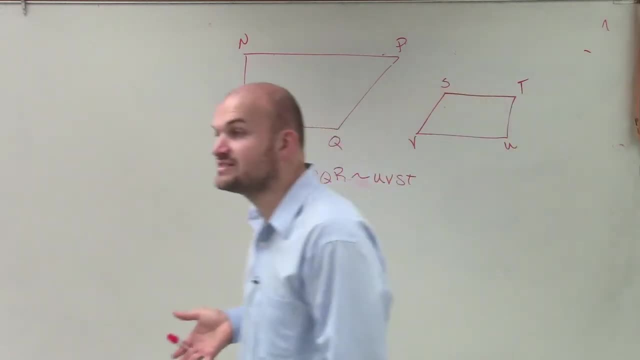 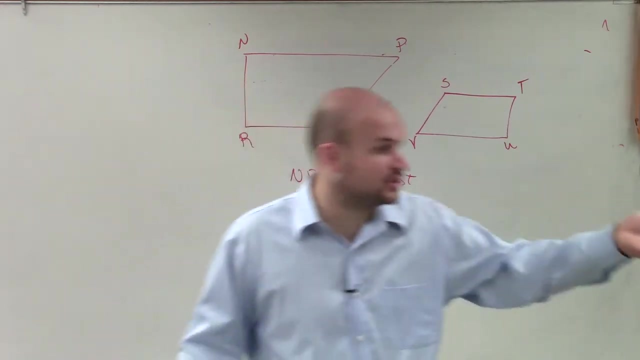 When we have similarity, one thing we want to do is write proportions of sides that are going to be similar to each other, as well as write angles that are going to be congruent. right, Because remember, when we looked at those two triangles that I helped you with right. 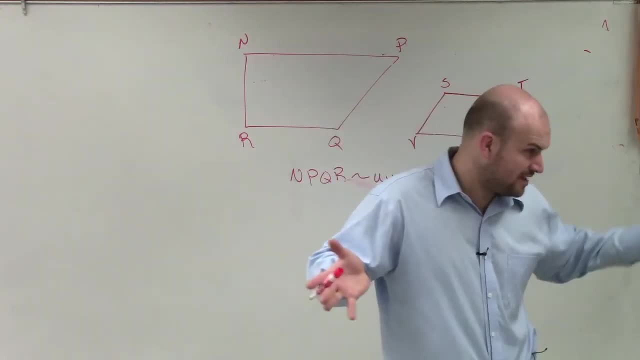 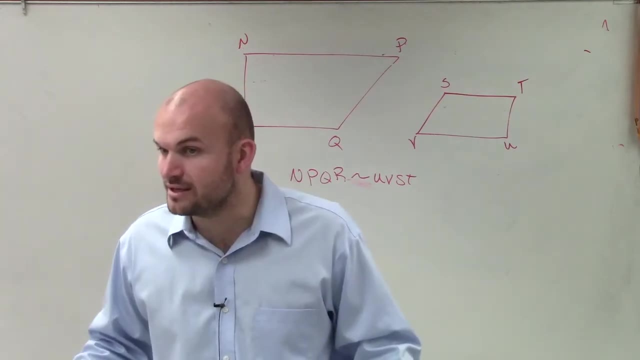 We knew the shapes were not the same size, right, But were the angles exactly the same? Yes, So when you have, the angles are still going to be exactly the same, meaning they're going to be congruent, But just because the angles are congruent. 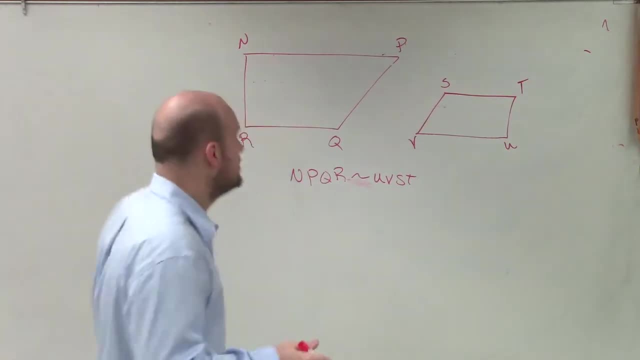 does not mean that the shapes are going to be congruent. So the first thing that I would want to do, guys, is write down my congruency statements for my angles. Now you guys can look at the figure, But also, if you're provided a statement, 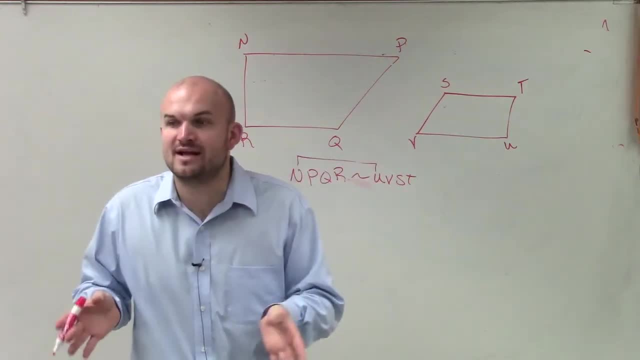 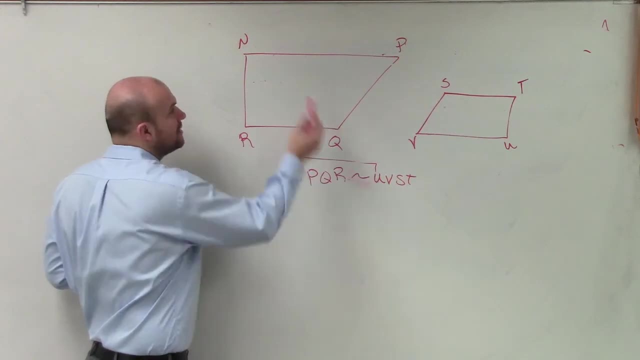 you can also just look at it, Remember, because when we write statements, we have to write them in congruent order of their angles. So therefore, n half is congruent to u. And look at n and u. Do those look like they're the same? 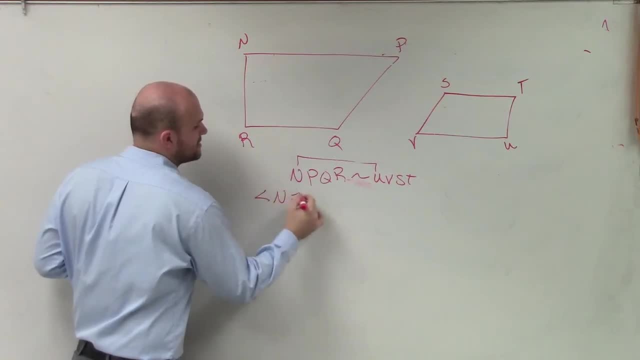 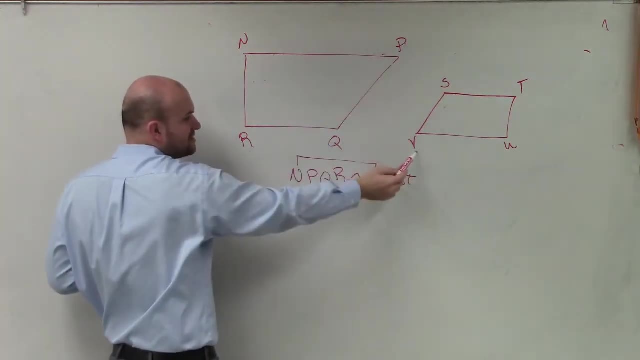 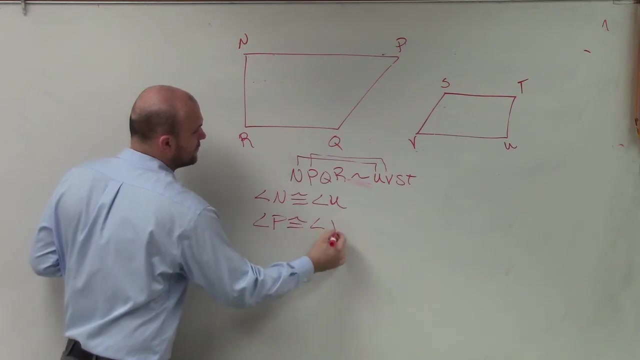 Yes, So I can say angle n is congruent to angle u. Then let's go to p. Are p and v? look like they're the same. Yes, So angle p is congruent to angle v, right? So it's very important if you have. 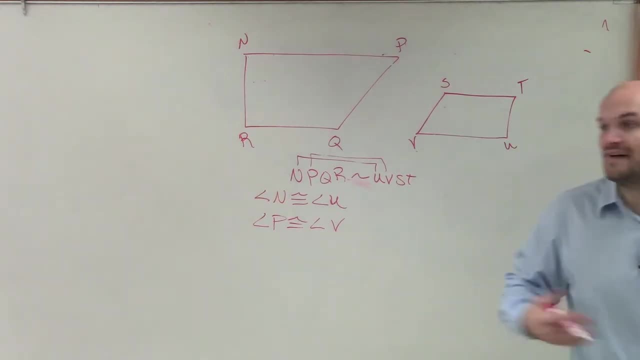 to write a similarity statement, or, if you're provided a similarity statement that already tells you what angles are congruent to each other, right, You can just follow along in the pattern. So angle q is congruent to angle s and angle r. 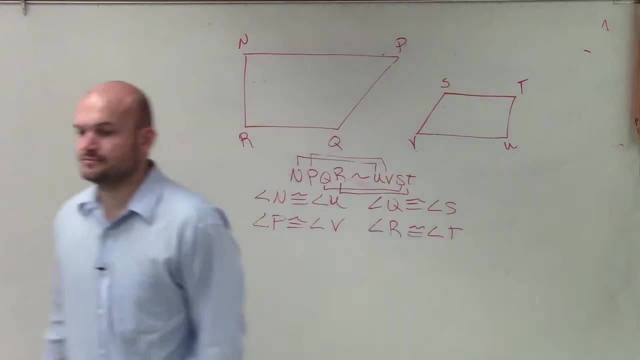 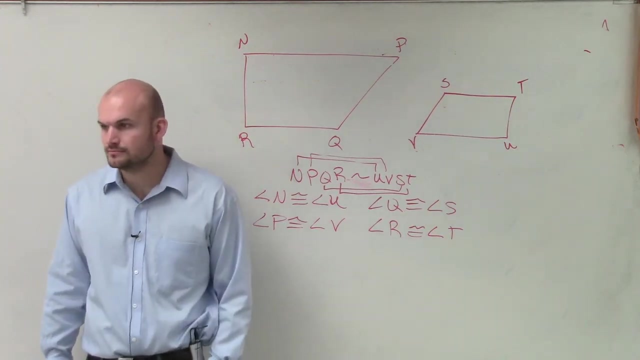 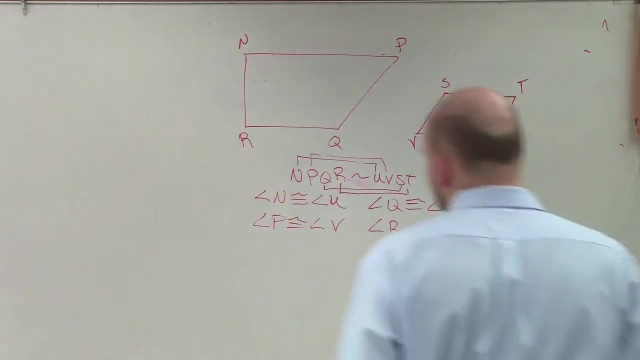 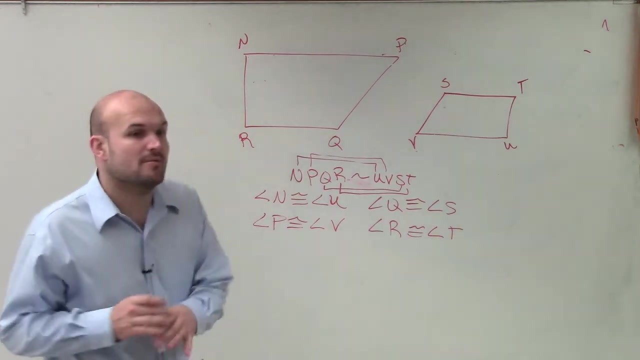 is congruent to angle t. So does everybody see that? Cool, Cool, All right. So now we're looking at that, And so now what we'd like to do is write a proportion for similarity. So remember, Caleb, when we were talking about proportions. 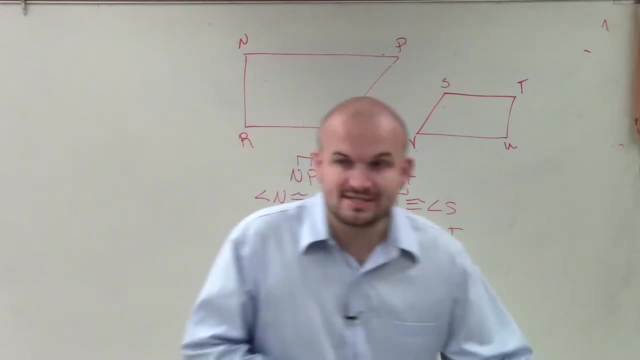 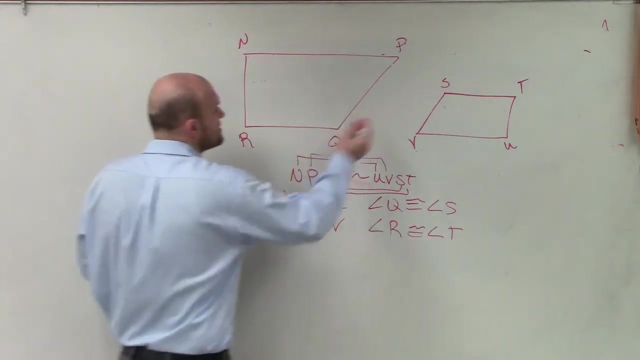 last class period we said it's a comparison right. One side is compared to the other, right. So what we're going to be doing is we're going to use fractions to compare them. But, Caleb, p q, what would you say? p q compares to. 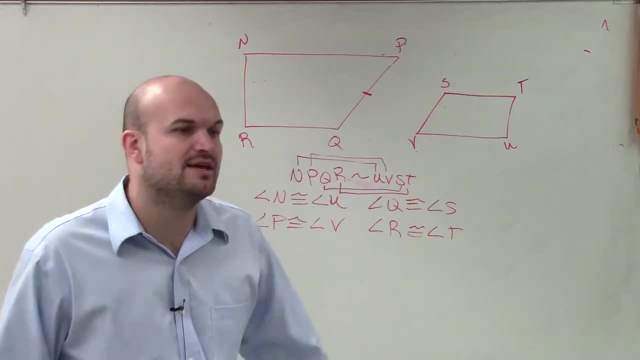 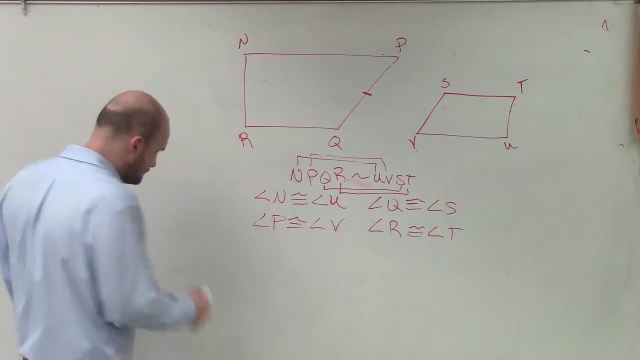 Which one of those sides in that other quadrilateral does p, q compare to To tu? Well, here let me give you a helpful hint. p to q is right here. Over which side would it compare to? over there, The s right. 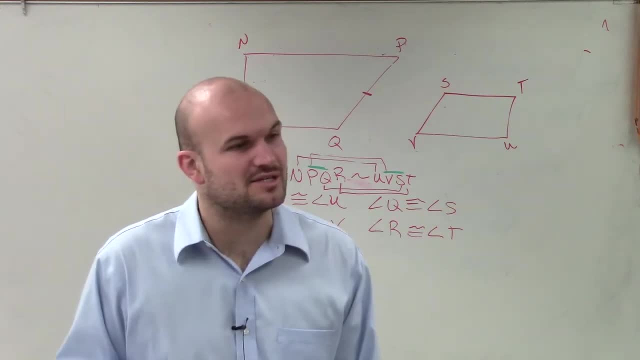 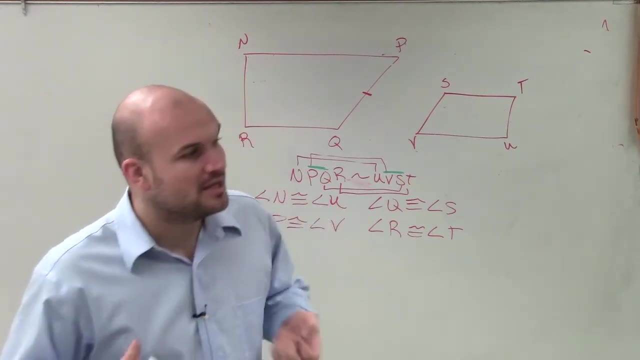 It's OK. But that's a very important thing, Robert, because a lot of times when you guys are doing these problems, you might get confused on looking at the figures right. The figures might try to mix you up. So one thing you guys can always do: 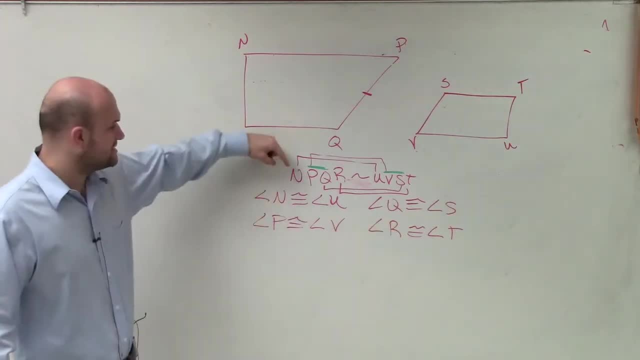 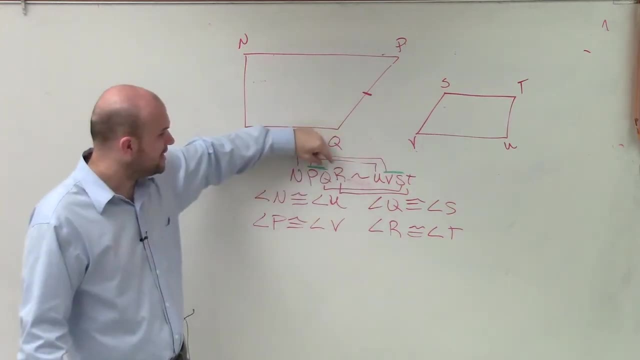 is go back to your similarity statement And what you can look at this is say: oh, np is going to be a ratio with uv, pq is a ratio with vs And qr is a ratio of st And then nr is a ratio with ut. 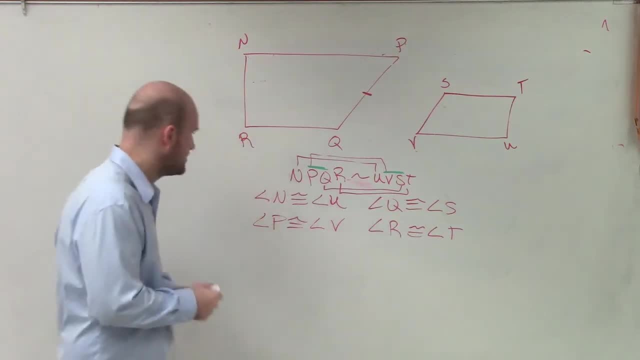 All right. So what we're going to do is I can now say with my ratios that np And p- this is the longest side right. Is that the longest side? What's the longest side over here? uv. So I could say np is compared to uv. 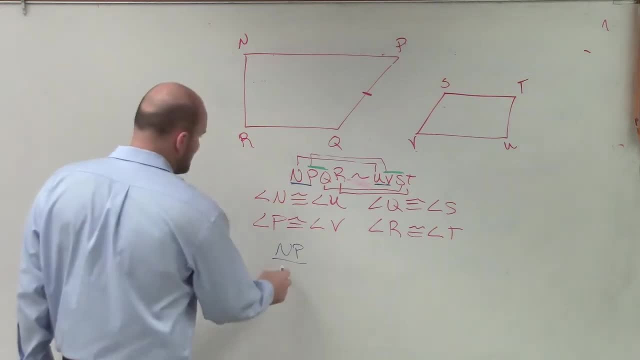 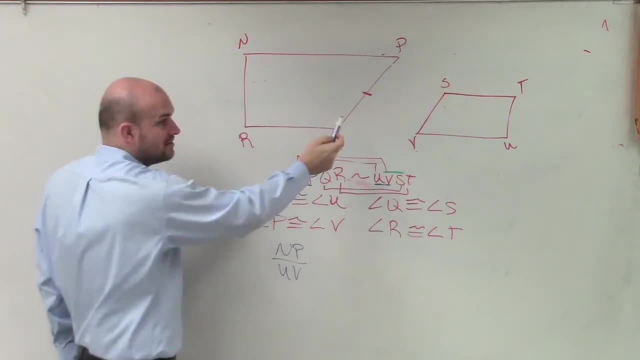 Does everybody see that? They're both the longest sides? So np is compared to uv, pq. pq is the only one that's slanted right. pq is the same thing as vs. Yes, Yes, OK, Oh, Oh. 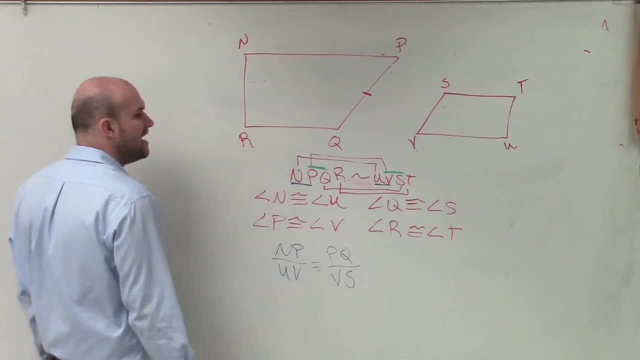 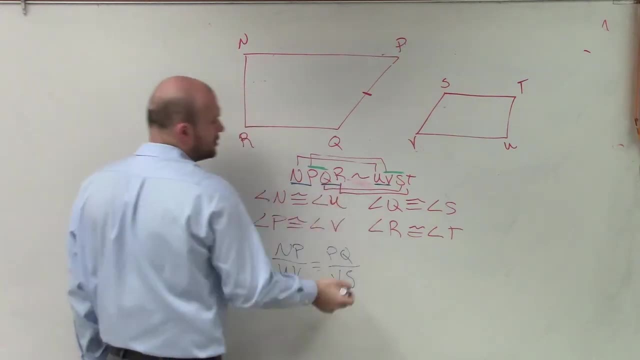 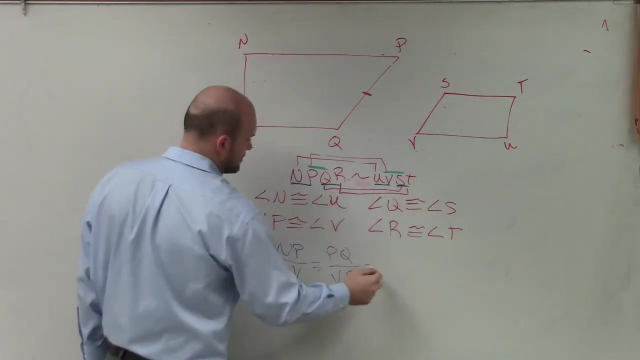 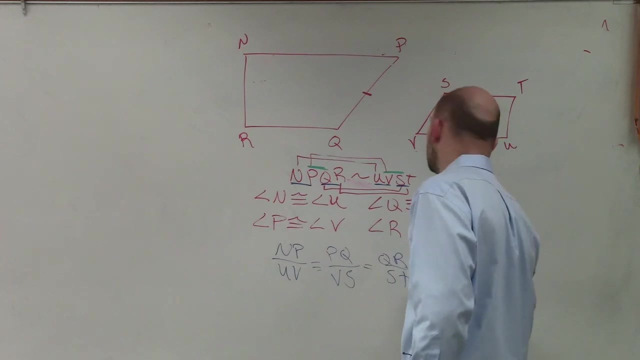 OK, Then we can go up to qr. qr looks like that's about one of the shorter lengths, qr should go to st, And then the last one I could do, rn, And rn can go to tu. OK, So what I'd like you to be able to do, 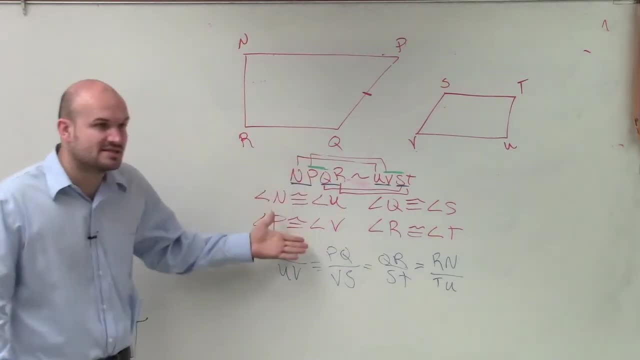 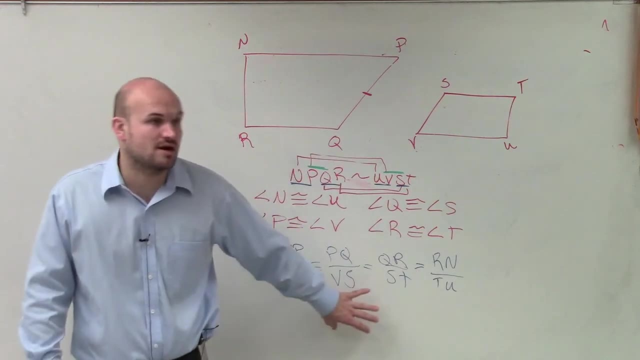 is, go ahead and write not only your congruency for your angles from your similarity statement, but then also write the proportions, Because that's going to be very important for how we're going to be solving these. OK, Write the proportions. How does one side from one figure relate to another side from the other figure, All right.